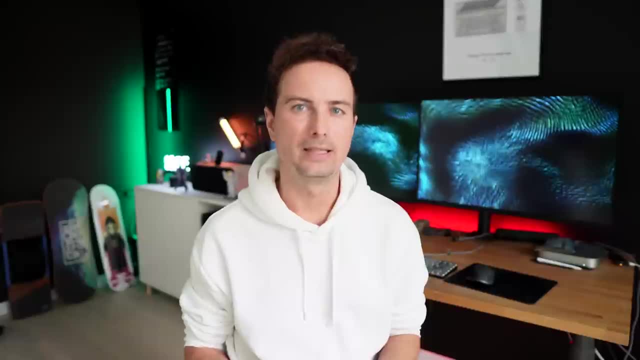 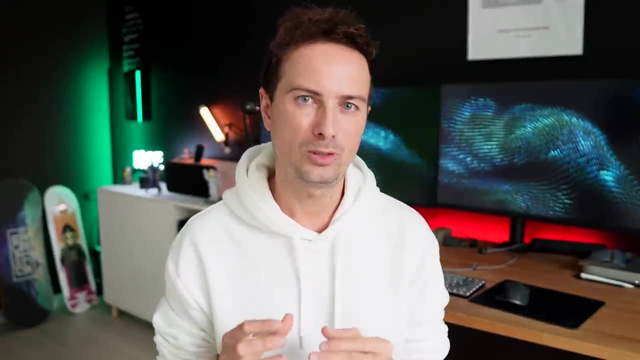 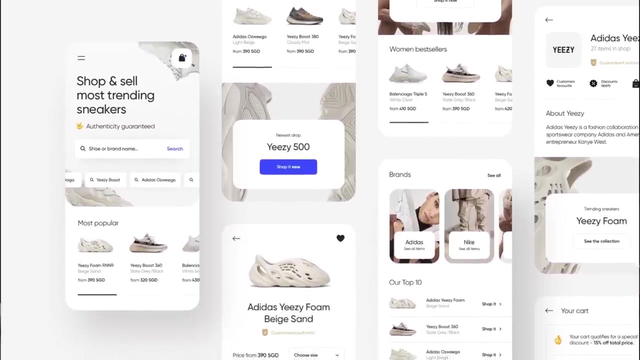 There are five main levels of UI design quality, and only level five is the one that you should be striving for. This is the level where recruiters will actually be reaching out to you directly themselves, without you chasing after them. We already established that for juniors you need. 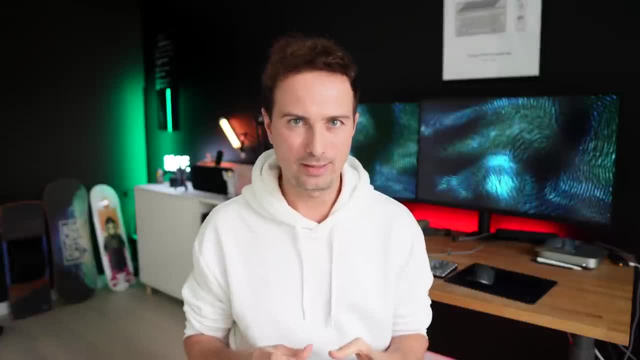 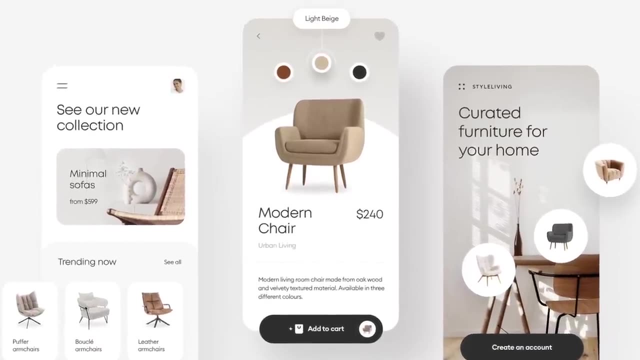 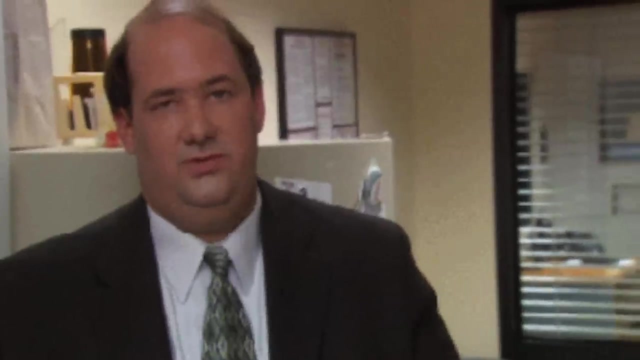 really strong UI skills to get hired. The reality is harsh and simple. Your UI skills grow the more you do it, the more you practice, based on the right learning sources. At level four you have a pretty big chance of getting a job if recruiters notice your portfolio And anywhere below level. 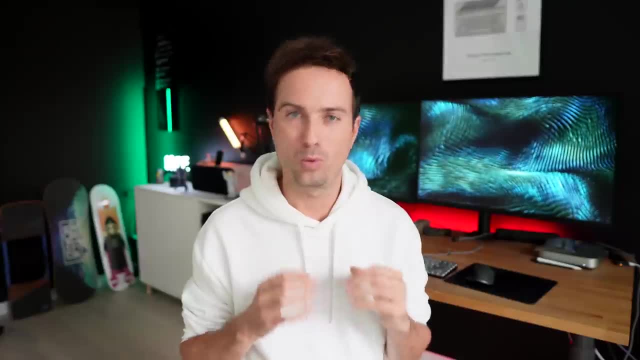 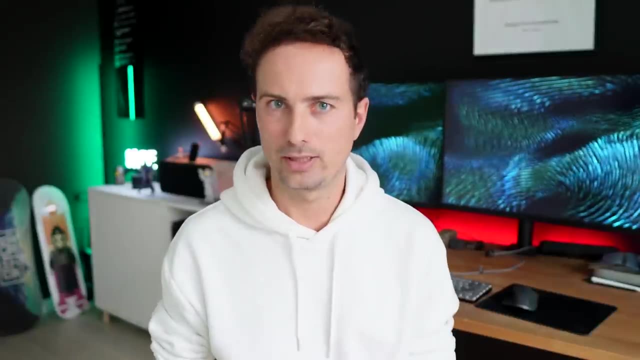 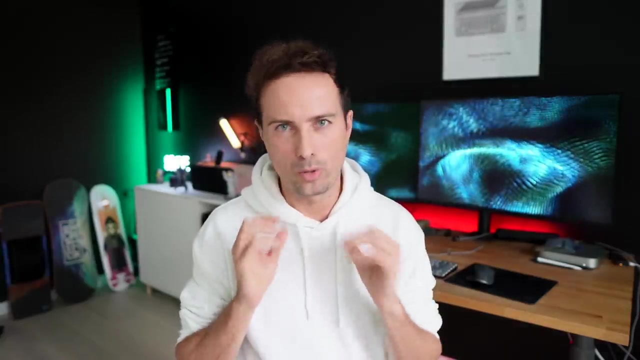 four, you need to be extremely lucky to get hired, or wow the recruiters with something else. The more you practice and the more you learn how to recreate great design, the bigger your chances of getting the industry job. Did I get the job? Yes, At level five, there's gonna be a lot of. 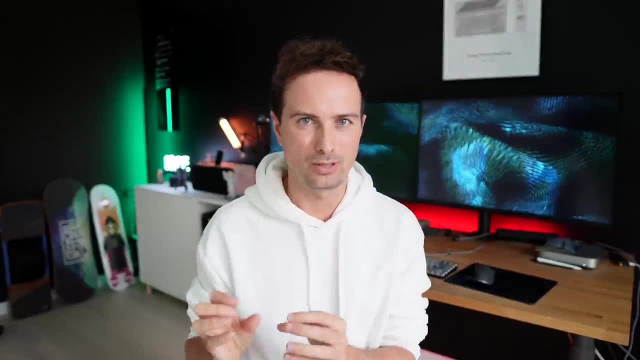 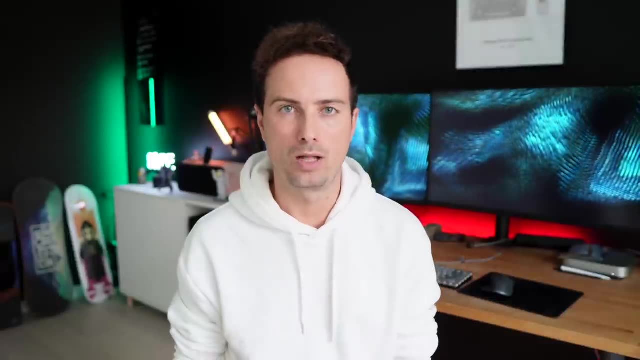 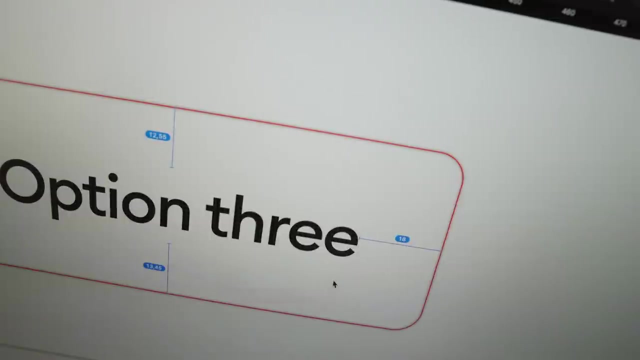 small, seemingly invisible tweaks and changes in the design that most regular people will never notice. That includes the recruiters in many cases as well. They won't know that you used a special golden ratio spacing distance here, but they will feel it because if the design is good objectively, 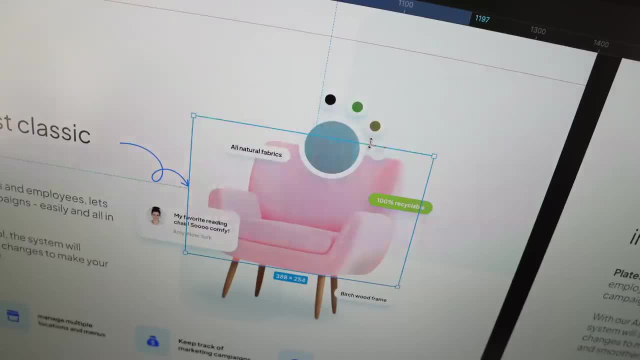 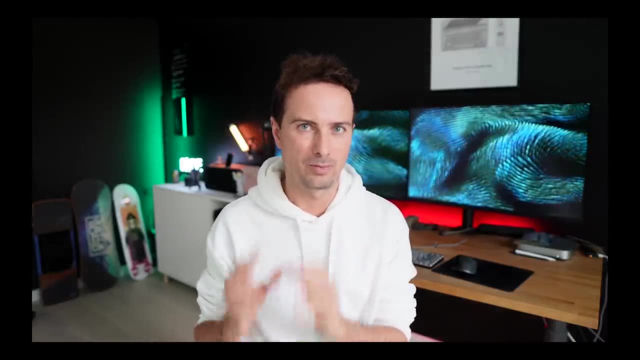 good and it's a pretty objective, measurable thing, then people subconsciously feel that it's something of high quality. In this video, I'll guide you through all five levels of app design. I'm gonna be using an app that we designed at level five and then I'm kind of 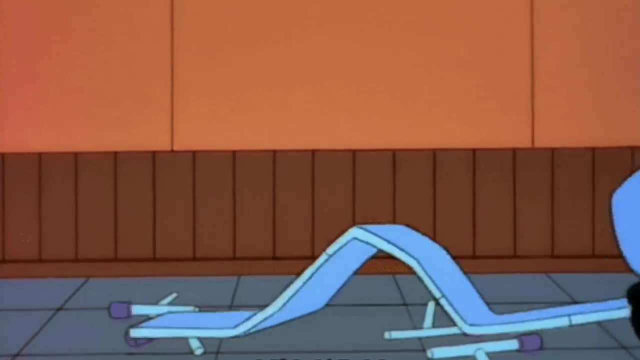 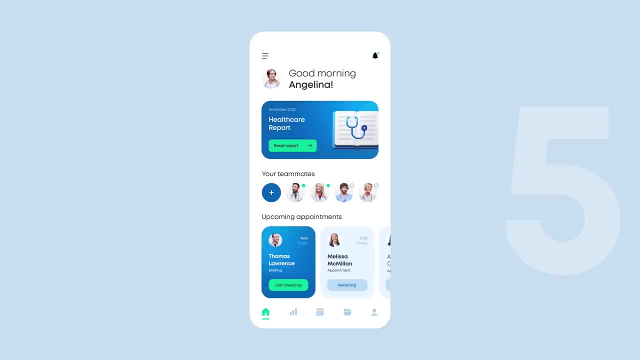 gonna try to break it a little bit for every level lower than five. We're starting with number five and keep in mind that, of course, this is just an example. A real product probably could look a little bit different and possibly even better, but this is to show you what an approach to a 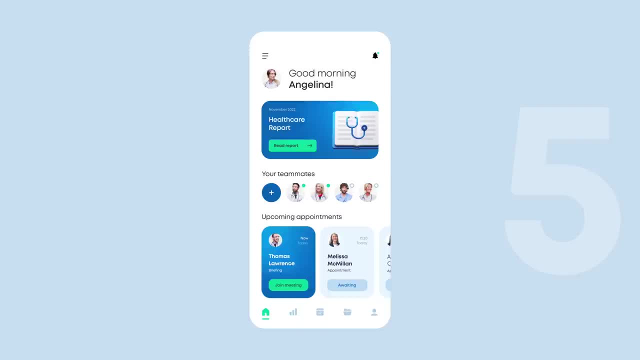 number five stage is: At first glance it just looks good, It looks dribble worthy, but is there more To it? let's explore One thing that's a dead giveaway of a good product is what's the font that the designer picked? How many different font styles are there? How many different font families? 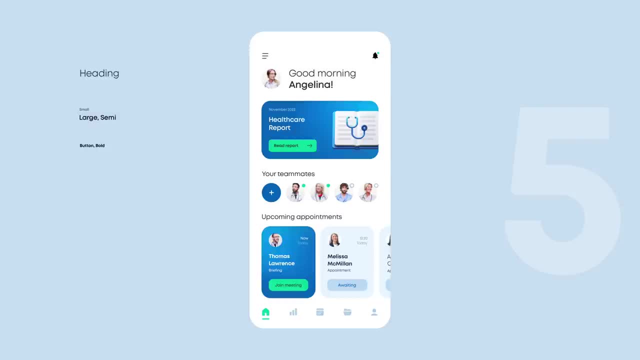 and font sizes And, as you can see, this design just has one font with four sizes and a couple of styles. All of the icons are not randomly placed, but rather they have their own invisible touch targets and they are aligned to those touch targets with regards to the rest of the 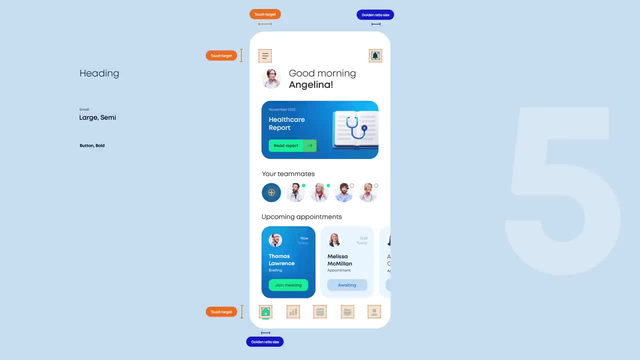 interface. Another thing is that the icons within the touch targets and the icon within the circular button, the plus, are not randomly spaced. It's all calculated based on some of the design principles and it can be calculated in multiple ways, but the point is that this is made that way on purpose. 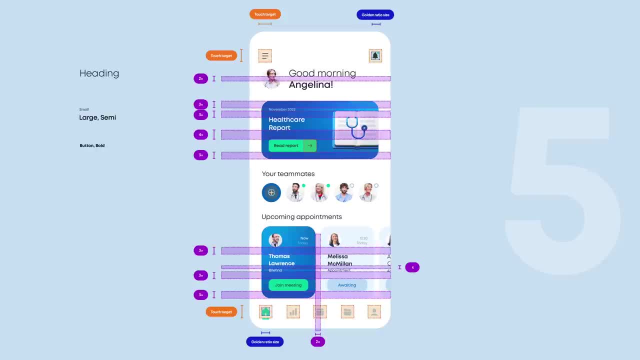 This is not a random size for the icons. Now, I'm not gonna show you pixel or point values here, because that's not the point. As you can see, we have an X on the right side of the icon. This is the base of our grid, and when you align everything correctly, you'll see that there are no. 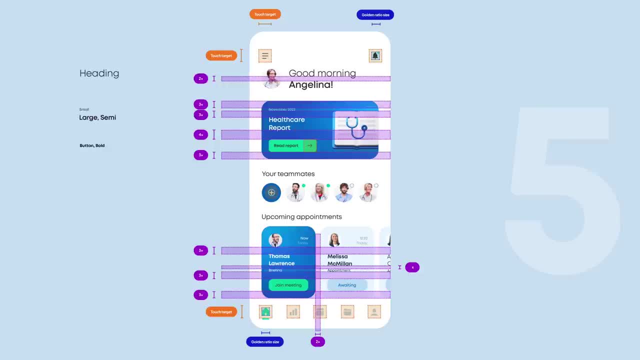 random values. There are multiples of X everywhere. That happens to practically every spacing from every side. Nothing is random here, And that becomes even clearer when we simply divide all of the objects in here, all the elements, into logical groups, As you can see. 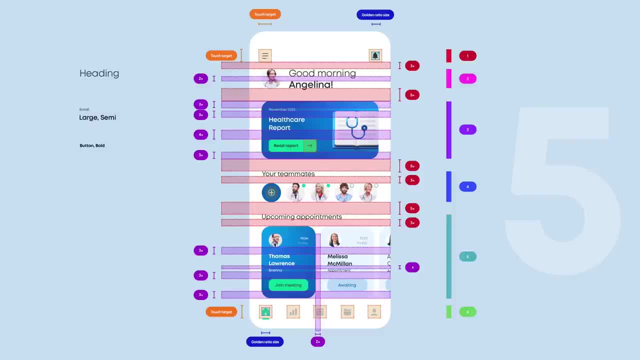 there are different spacings between the groups, but they are consistent. That way, we can the entire screen and quickly understand which element is belonging to which section and what is connected to what. This is the basic and the principle of good UI design, And I'm not gonna even mention the obvious things like consistent corner radiuses and 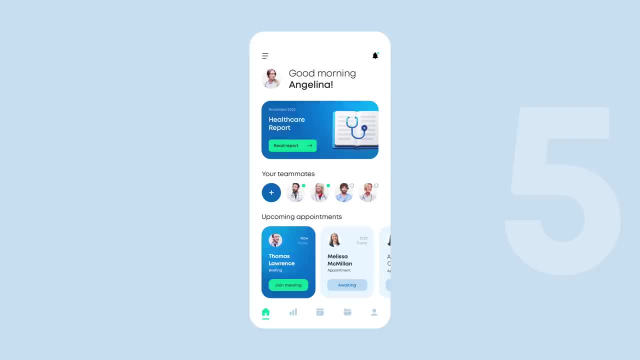 consistent spacings on every side for buttons and other on-screen elements. One thing that is also important to mention is consistent icon thickness for all icons that are outlines. This is stage 4.. It's actually still a pretty good design. There are some small issues there. 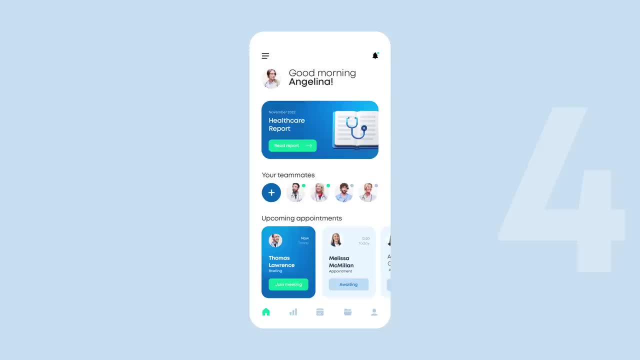 but if you can make designs on that level, UIs on that level, you shouldn't have a problem with finding a job. But let's explore some of the differences between this and number 5.. The first thing is inconsistent icon thickness and, as you can see, this one icon that I'm pointing. 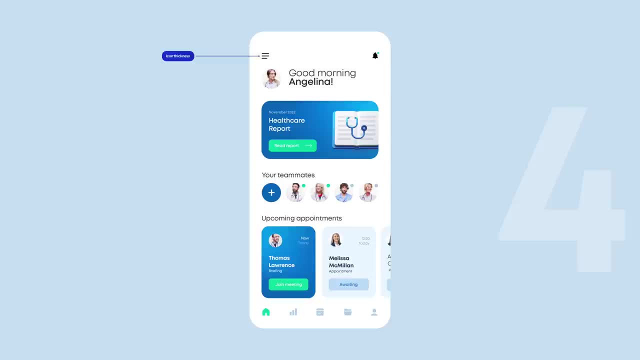 at right now is of different thickness than the arrow on the button and some of the other icons on the screen, Cause, yeah, the icon on the button is too thin, especially comparing to the thickness of the font on that button. Someone was going fast here and there is slightly. 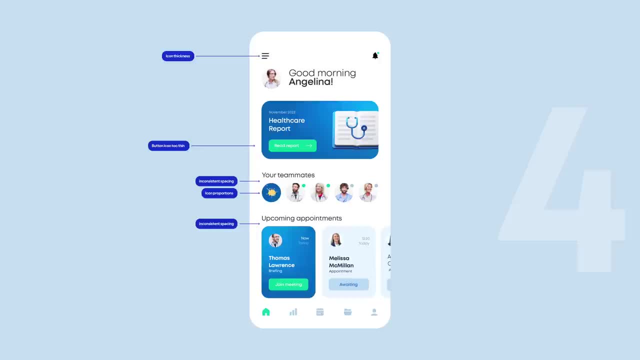 different spacing between very similar looking headers. The plus icon size was, I think, just id and wasn't really calculated. It's not really bad, but it's not really matching the aesthetics of the entire design. And here's somebody also forgot that using color alone to 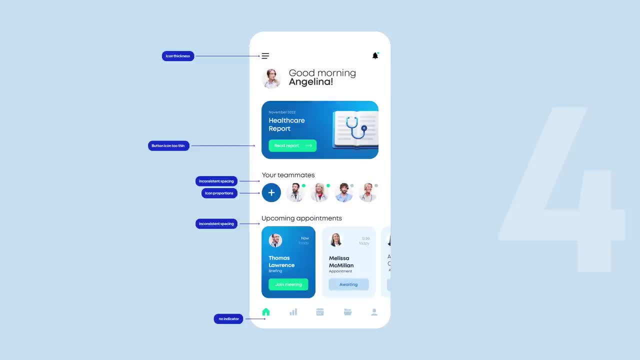 the selected tab is not enough, because some people won't see that color, so you need at least to have some sort of an indicator or a background that's different so it works for everybody. and similar thing here: the inactive indicator is just a slightly different color than the green, but it 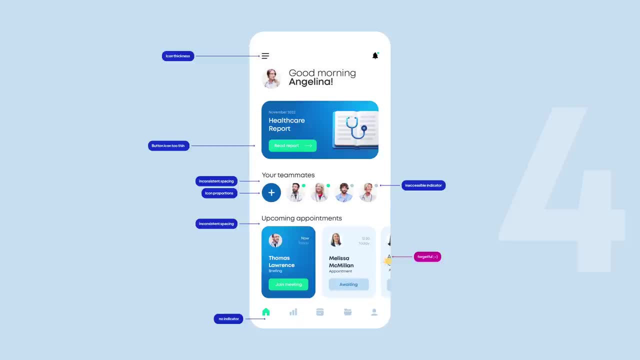 doesn't look different for people who won't see the color, and this is something i find extremely funny, actually, because when you're making a design like that, you often come up with different versions of the cards and you sometimes forget that one of the cards. that's just a little bit. 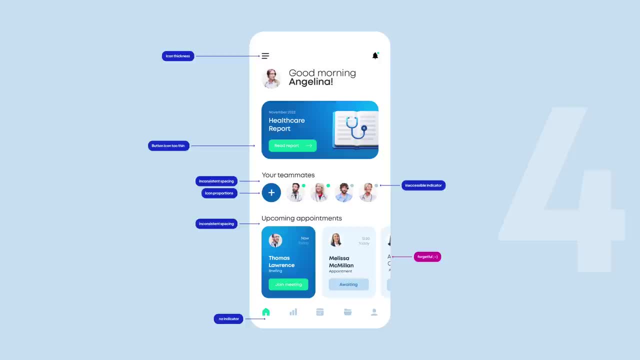 sticking out from the side of the screen has still different font sizes and a slightly different alignment, because, yeah, nobody notices that right. and when we add the calculated spacing from stage five, you'll see that these spacings are not as calculated. things are a little bit randomly spaced. 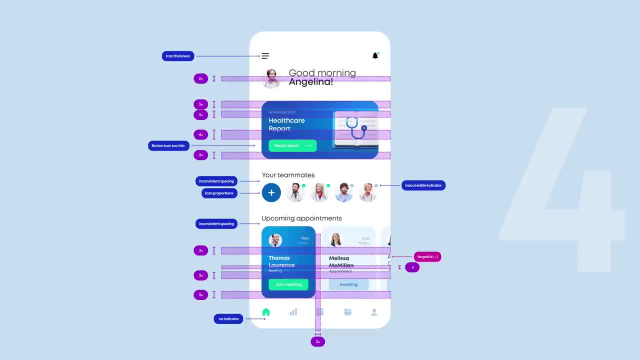 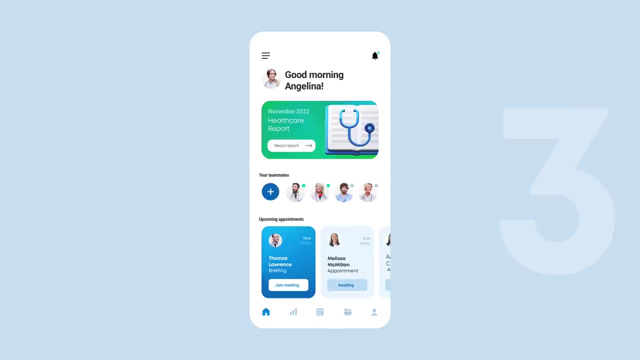 the still look pretty good, but it's not really based on anything. so a lot of the visual hierarchy is broken and the groups are looking a little bit different now and if you have a ui design on that level, chances are you're still gonna get hired for a junior role. welcome to level three. 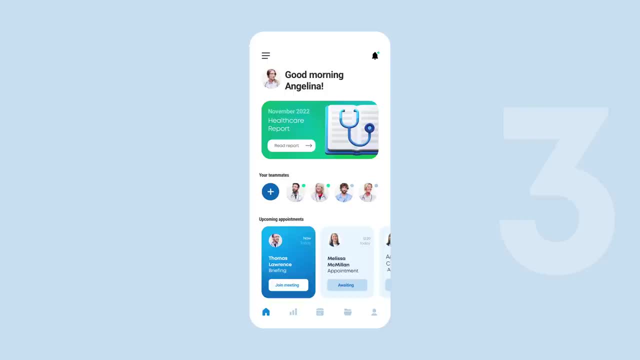 if you're at this level and you've been designing for less than a year or around a year, congratulations. this is a good place to be, but this is not a hireable level. the first issue is what a lot of people say is that it's too cumbersome to just be qualified. what's the next step? 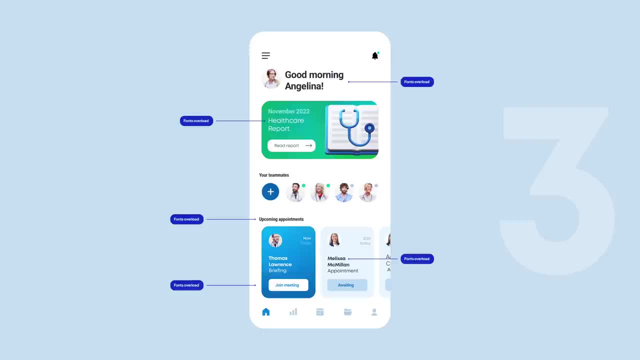 so the next step is to start by creating a writing style for the app and for the font. so it's not really a problem to start with a font font, so let's start with font font. you can start by creating a font name, so let's just start with font font. art mode. 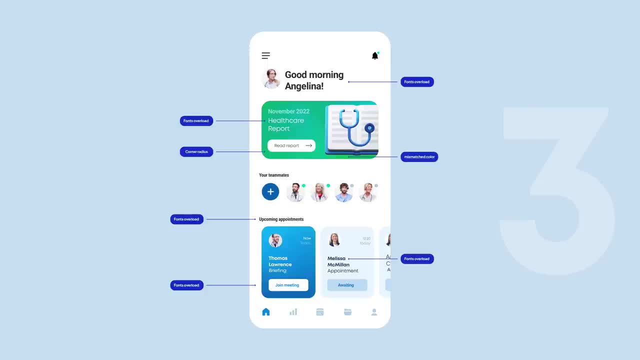 we can use font typo and other font types, but let's just for thefestive start with font type color, which is what i call font overload. there are a couple different sans serif fonts in here and too big and not proportional to the content. There's also chaos in text hierarchy because 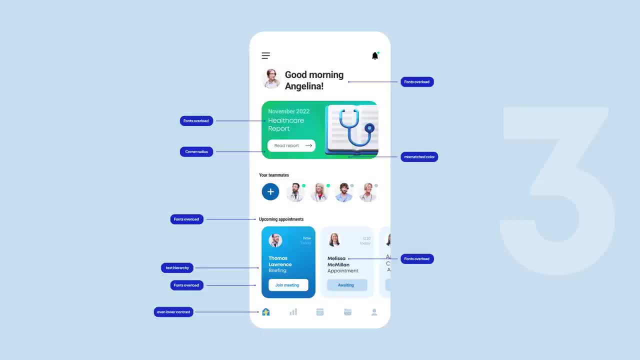 it's too big and too close together, It's really hard to read. The bottom menu selection has an even lower contrast. Practically everything on this screen is misaligned and a little bit mismatched. A good example is the heading font being too low and the plus circle being a little. 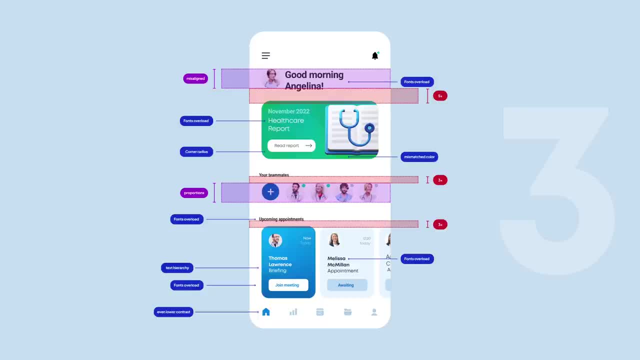 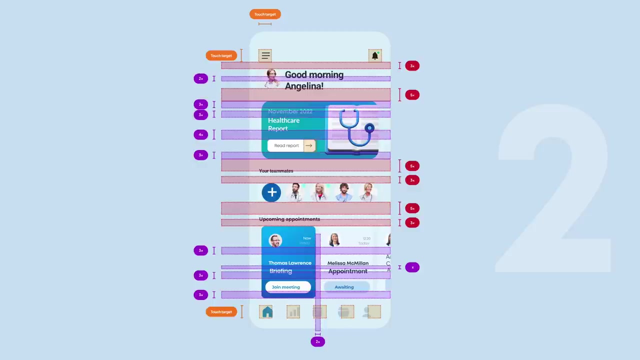 bit too small, considering how big the icons next to it are. At first glance it doesn't look too bad, but it's really far from an employable level design. Welcome to stage two. If you're at this stage, you still have some work to do. Just looking at the alignment, practically everything. 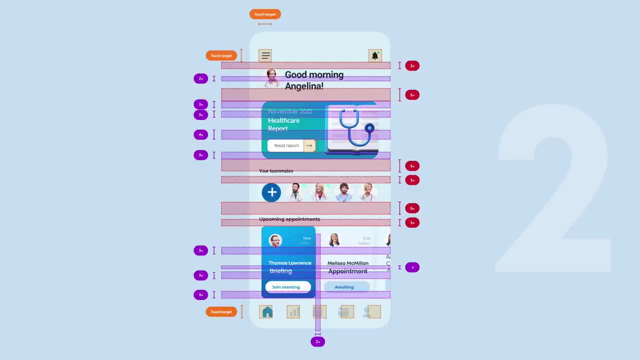 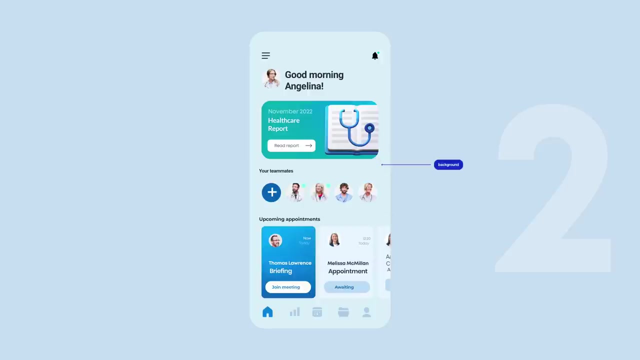 is a little bit off, misaligned, moved to the side and not in the right spot. A good example is the bottom navigation icons, which are too big and align pretty randomly. Also, trying a colorful background when you're just starting out is really risky and you can end up with 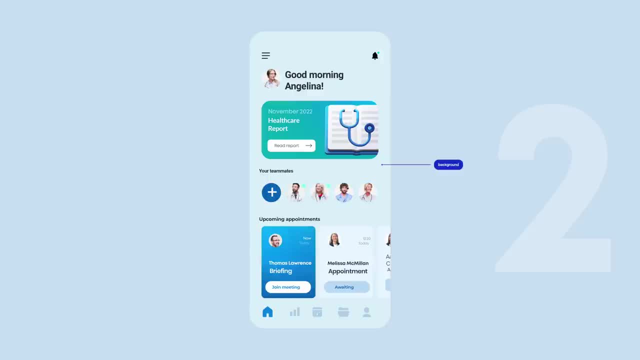 something like this that doesn't really match any of the elements on top, Classic font overload with different spacing, misaligned fonts and different font styles even between similar sections. On top of that really bad alignment and in oh, so many places, That background indicator. 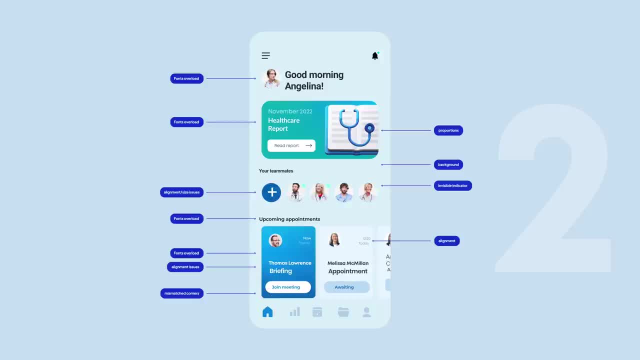 is barely visible. The 3D illustration proportion inside the first card. yeah, that's really, really bad, And even here we're still pretty forgetful. If you're at stage two, keep going. You're already doing some things right, but there's still a lot for you to learn And you can. 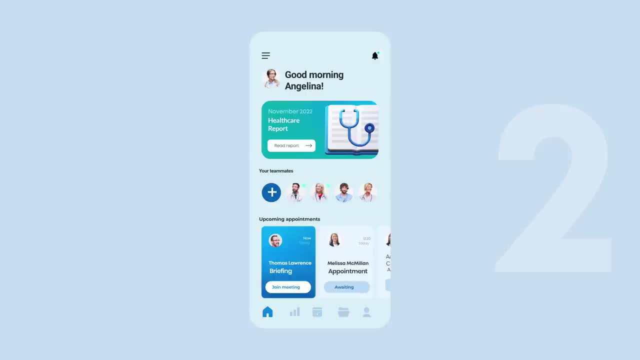 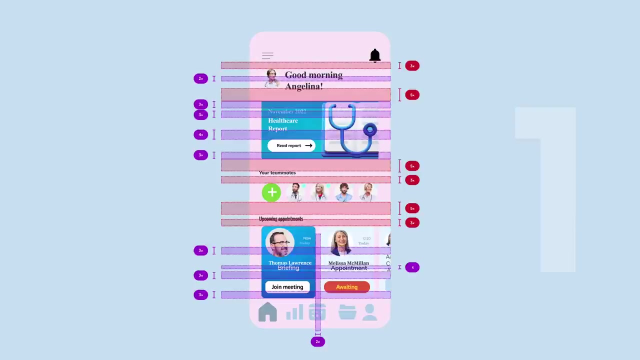 learn a lot of that from my YouTube videos and my courses And leaving the best for last. As you can see, pretty much everything that can be wrong is wrong here. Two big icons missing, touch targets completely misaligned, everything. multiple different fonts with different spacing, multiple. 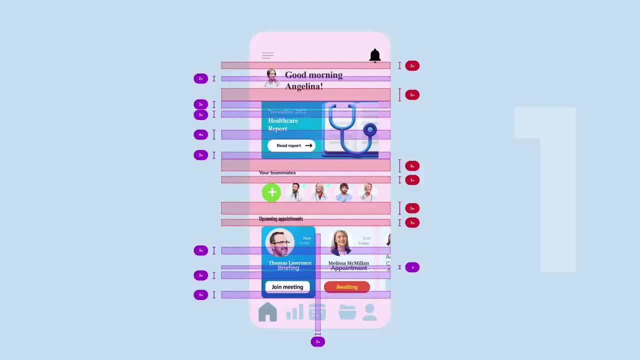 radiuses, different line thicknesses, different colors and a background that doesn't match anything here. If you're at this stage, you have a lot of work ahead of you, But don't worry, because that shows that you know how to move some rectangles, So now you need to move them.